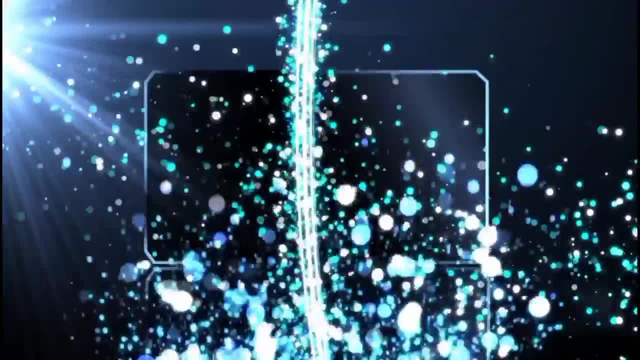 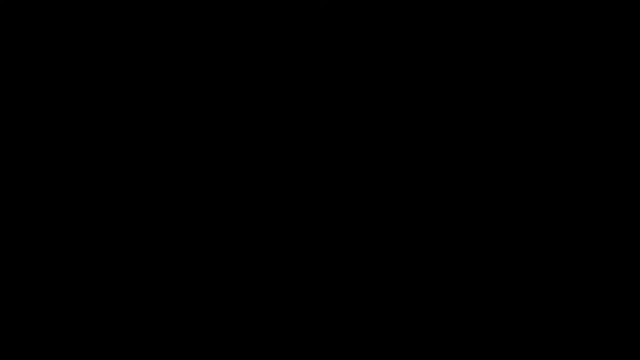 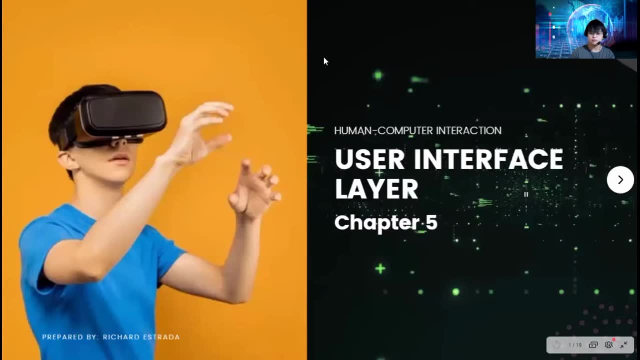 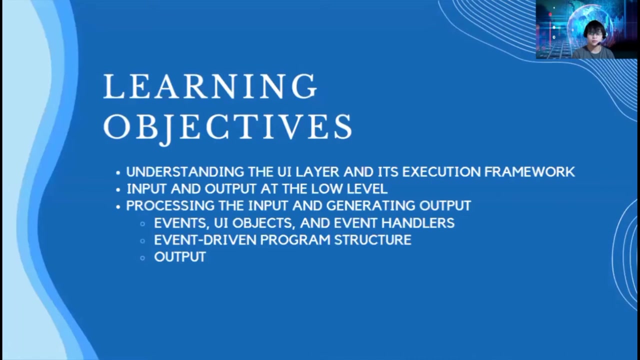 Hey everyone. and we are now in the chapter 5 of human-computer interaction. So for this chapter, we will be learning and discussing about the user interface layer. Okay, So these are our different learning objectives. First is we're going to you. 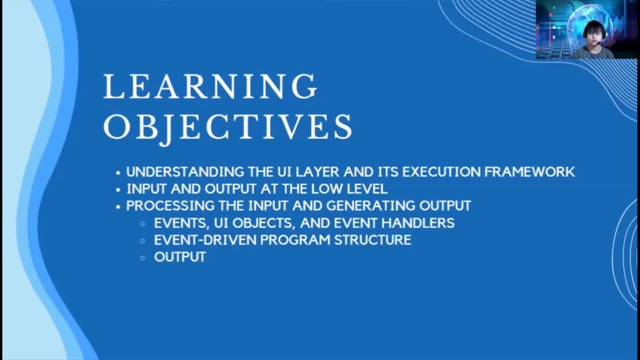 know understanding the UI layer and its execution framework and what are the? the input and output at the lower level and they're processing the input and generating output. So we will be discussing about the events, UI objects and event handlers, event-driven program structure and the output. Okay, So, 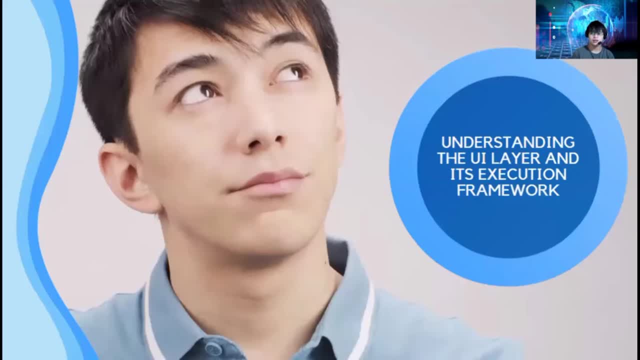 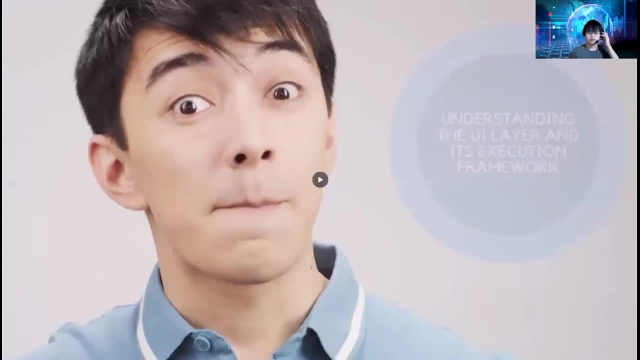 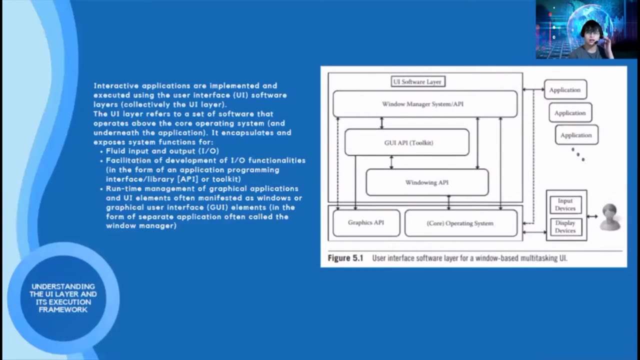 we'll start with understanding the UI layer and its execution framework. Okay, So, sorry guys for the font, It's too small. Interactive applications are implemented and executed using the user interface software layers, or, collectively, the UI layer. Okay, So the UI layer is a. 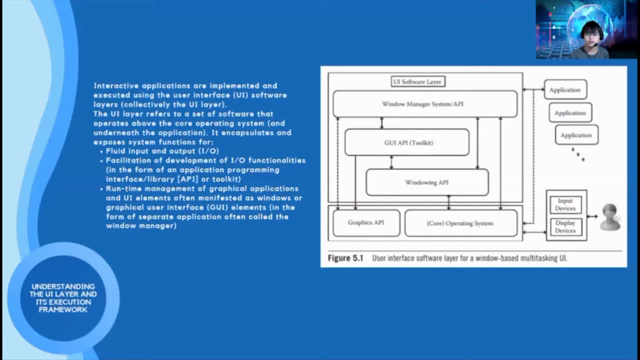 set of software that operates above the core operating systems and underneath the application. It encapsulates and exposes system functions for fluid input and output. facilitation of development for input output functionalities in the form of an application programming interface or library, API or toolkit. So 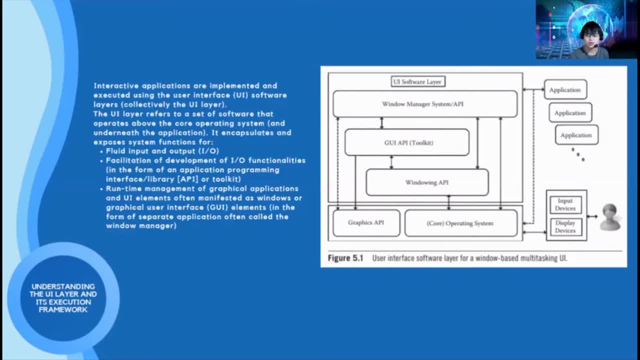 runtime management of graphical applications and UI elements, often manifested as Windows or graphical user interface or GUI or GUI elements, So in the form of a separate application, often called the window manager. So we'll discuss more about this figure, The figure 5.1.. Okay, 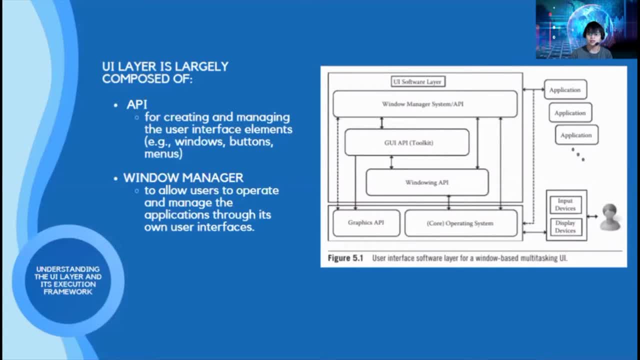 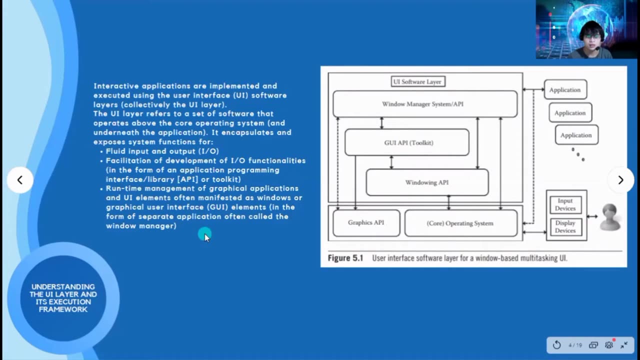 Before that UI layer, guys, is largely composed of APIs. So when we say API, it is the application program interface. I think I have attached the meaning of API here. It is the application programming interface or library. It actually is somewhat like a bridge between your application and your. 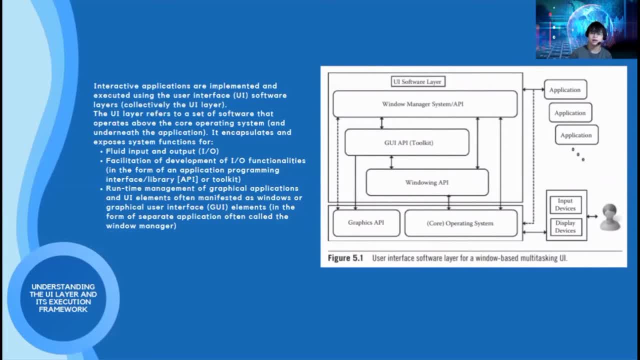 database. Now the API will gonna help us. It will gonna help you to access the data from your database sent to your application. Okay, So basically, this is a user interface that성이 operator that is always game on the Cloud. This API works very special for the applicationular. 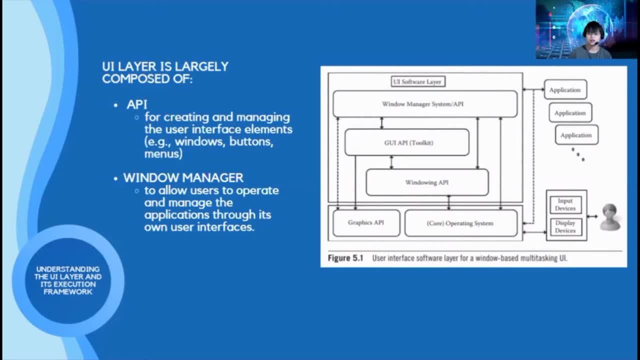 containers to make sure everything's running, sourced and Done. And then this user interface is going to allow the user to apps and normally run applications over a 내�ed, depois That applicants needyears to use virtual applications or to the user interface. Okay, So API is used for creating. and managing the user interface elements such as Windows buttons, revenues and etc. as you can see in this image. So the API is in this layer. So the window manager is to allow the users to operate and manage applications through its only user interface. so that is the Bible and it depends Galaxy as the context for the thing that you are looking for. So the API is driving the user interface itself and it is used by ground beds and it is created by long Jaw스트� to it in a basic package, so that we are forgot. architectше. 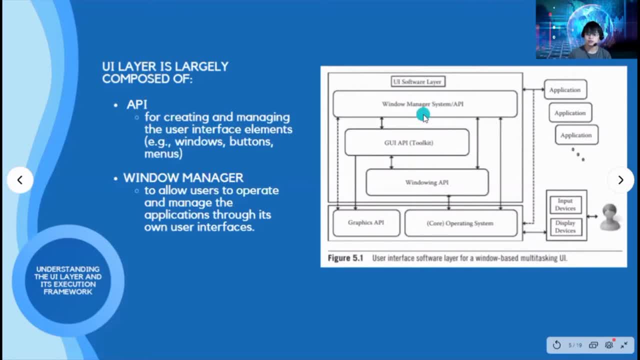 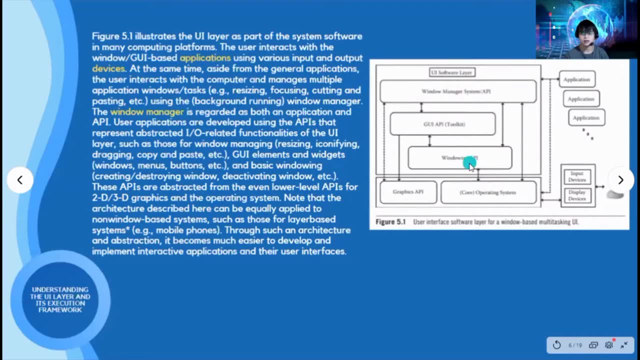 um, that is the window manager. okay, so let's discuss this. i know this image further, this diagram. so the figure of 5.1 illustrates the ui layer as part of the system software. okay, in many computing platforms. so the user interacts with the window or goi based applications. 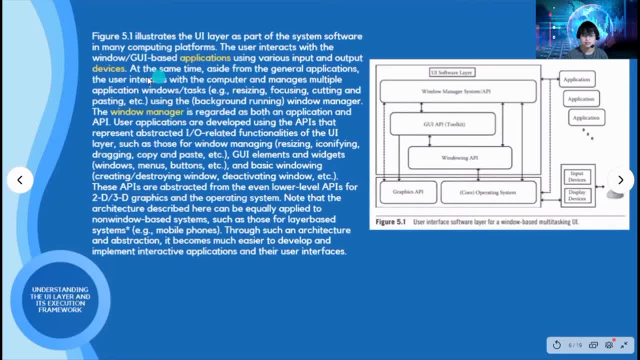 using various input and output devices: okay. at the same time, aside from the general applications, the user interacts with the computer and manages multiple application windows or tasks that could either be resizing, focusing and cutting or pasting. okay, using the different background running window manager- so the window manager is required- is regarded as 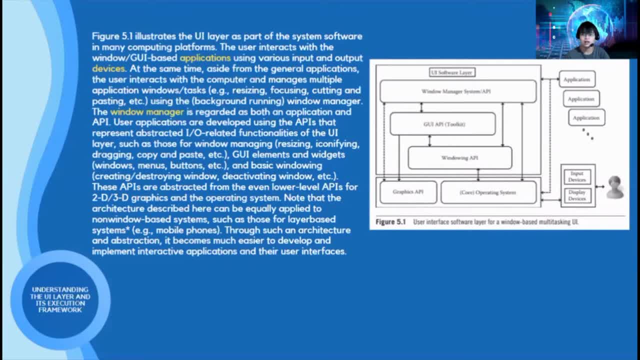 blocker, both an application and api. okay so, user applications are developed using the apis that represent abstracted input output related functionalities of the ui layer, such as those for window managing, or that could either be resizing, iconifying, dragging, copy and paste, etc. okay so, goi elements and widgets, windows menus, buttons. 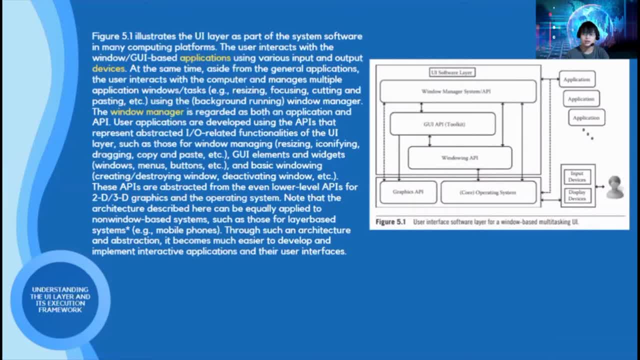 and basic window windowing or creating or destroying window, deactivating window, etc. so these apis are abstracted from even lower level apis for 2d or 3d graphics in the operating system. okay, note that the architecture described here can be equally applied to a non-window-based 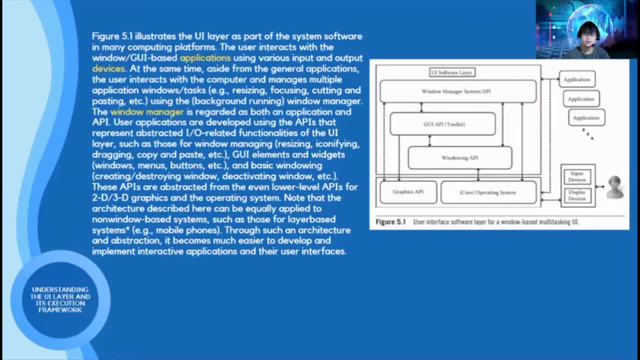 systems such as those of the layer-based systems samples. we have the mobile system, we have the mobile phones, so through such an architecture on abstraction, it becomes much easier to develop and implement interactive applications and their user interfaces. so again guys, um, the ui layer is always a part of a system, software in all computing platforms. so, as you can see in here, and so that is. 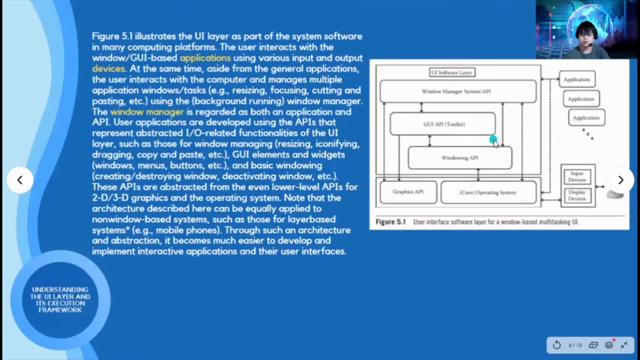 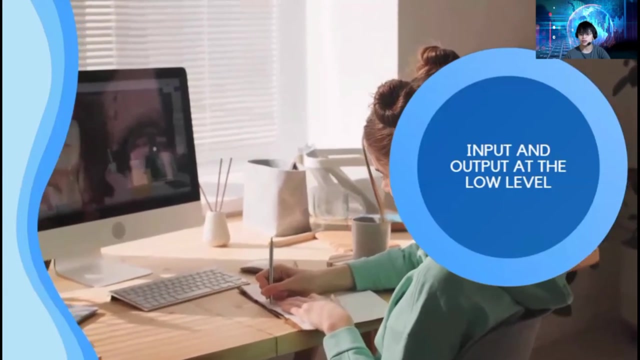 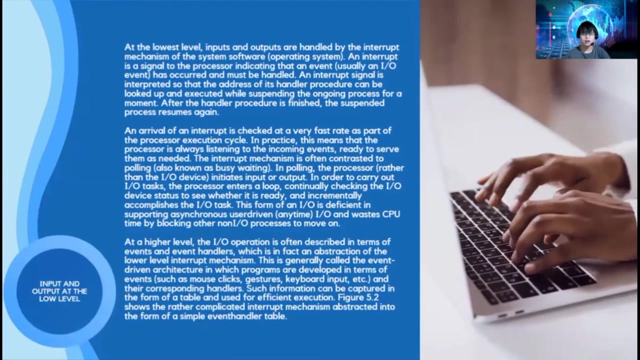 this figure illustrates. so user interface software application for a window based multitasking ui. okay, so that is the process. that is how the ui layer and you know its execution framework. okay, next is we will discuss the input and output at the low level. so again at the lowest level. 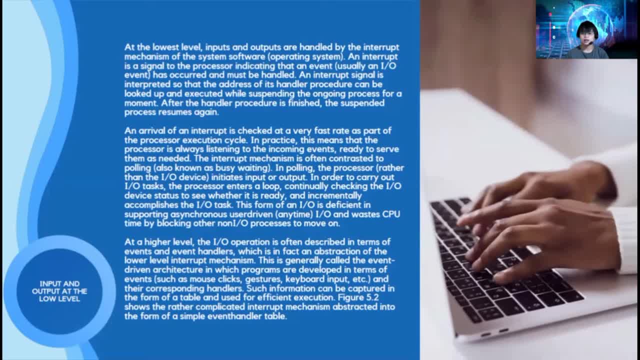 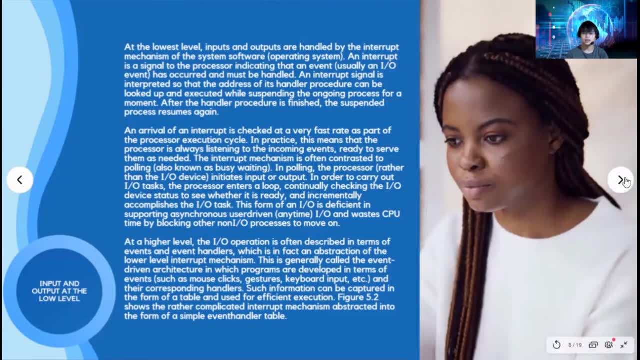 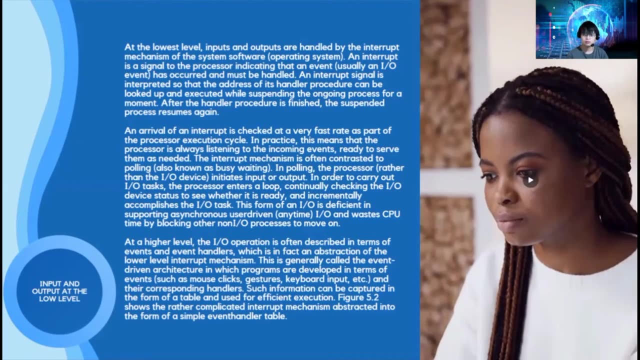 guys, um, you may have noticed the tag us on my text signing a presentation. it's because, um, um, i included the the discussion. um, um, um, um, um, um, um. you just know that the input and output at the low level, at the lowest level, inputs and outputs are handled with interrupt mechanism of the system, software or operating system. 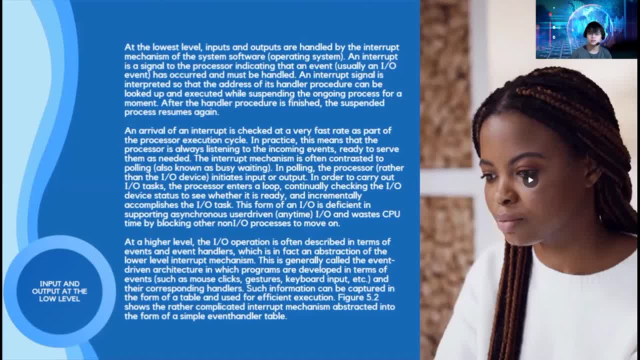 okay. so an interrupt is a signal to the processor indicating that an event Tilliembre 60 year vent- usually an input output event- has accord and must be handled. so an interrupt signal is enter hindler personal visits. which love how. that was what this sustainability capacityакс a marriage. 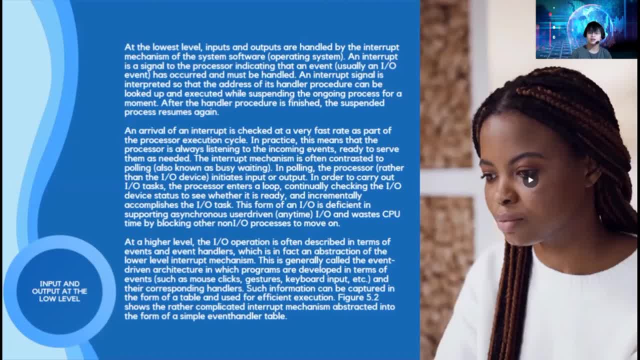 and life order allowed me to locked up and executed while suspending the ongoing process for a moment. so after the handler procedure is finished, the suspended process resumes again. okay, so again, guys, when you actually give instructions to a computer, there is what we called an interrupt mechanism. now that will you know a signal indicating 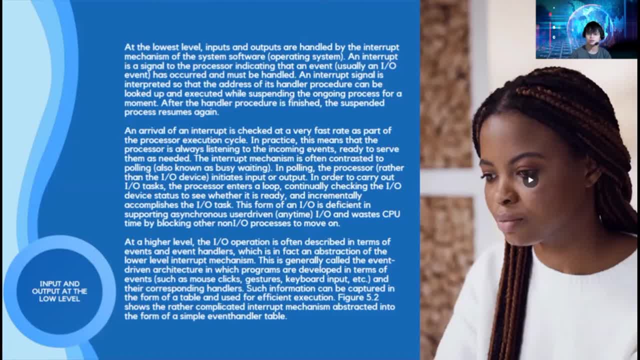 that there is a process now, night process. no button on your computer, okay. so an arrival of an interrupt is checked at a very fast rate as part of the process or execution cycle. so in practice this means that the processor is always listening to the incoming events, ready to serve them as needed. so 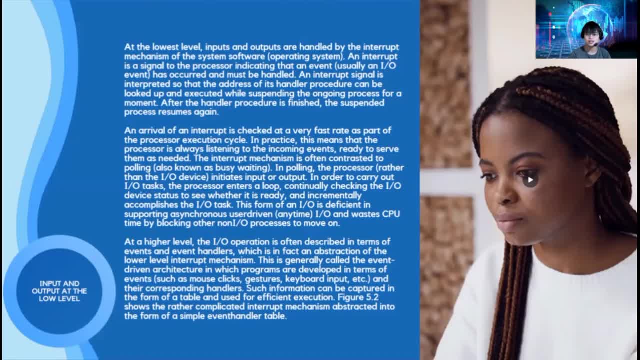 the interrupt mechanism is often contrasted to pulling, also known as basic waiting. so in pulling guys, the processor, rather than the input output device, initiates input or output. so in order to carry out the device status, to see whether it is ready, and incrementally accomplishes the IO task or the input. 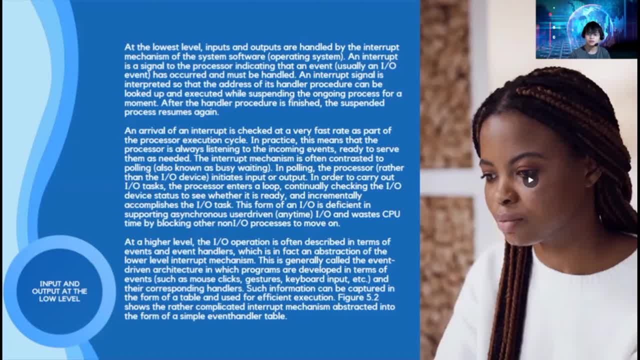 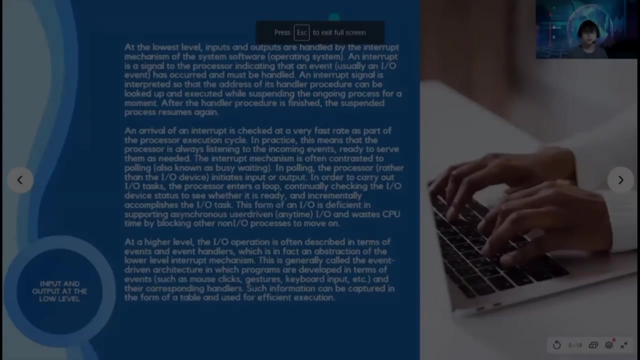 output task. so this form of an input output is deficient in supporting a synchronous user driven any time IO and wastes CPU time by blocking than other non IO process to move on. so imagine, imagine how, how it goes. no, so imagine how you know how amazing it is. so, at a higher level, the 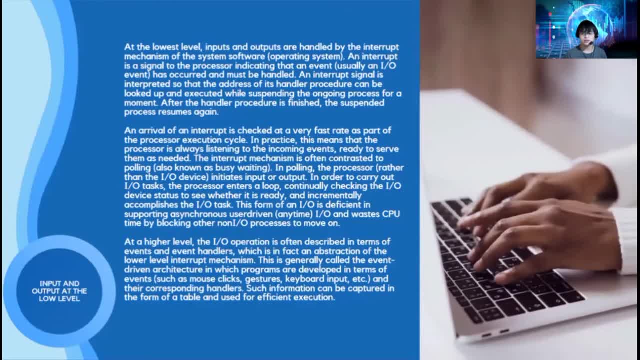 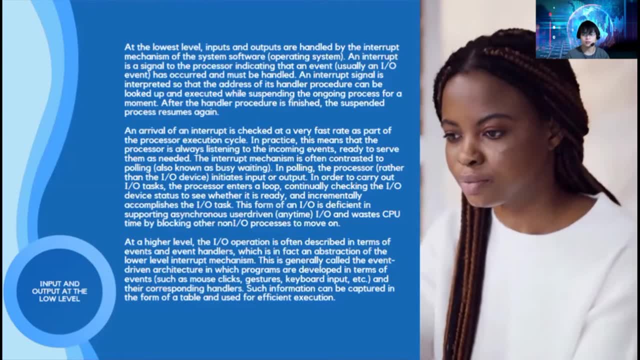 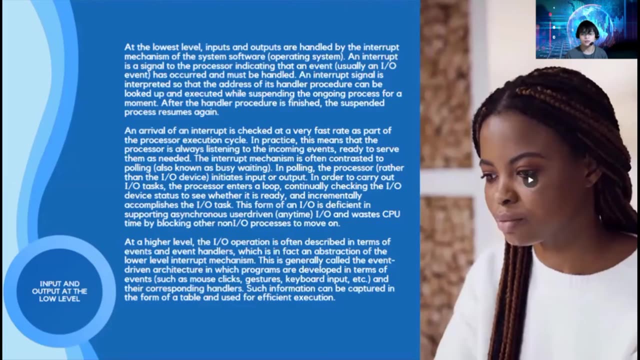 input output operation is often described in terms of events and event handlers, which is in fact an abstraction of the low-level interrupt mechanism. so this is generally called the event-driven architecture, in which programs are developed in terms of events such as mouse click and clicks, gestures, keyboard input and etc. and there's course and their 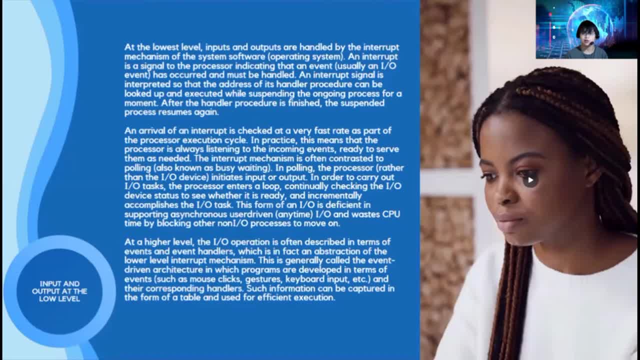 corresponding handlers. so when you are, you know, giving instructions to the computer, it created an event, the event that has event handlers. okay, such as you know, when you click on the icon, when you drag the icon, when you copy or paste and etc. okay, so such information can be captured in the form of a table and used. 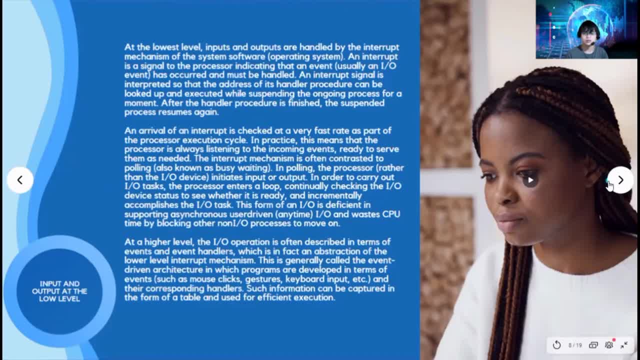 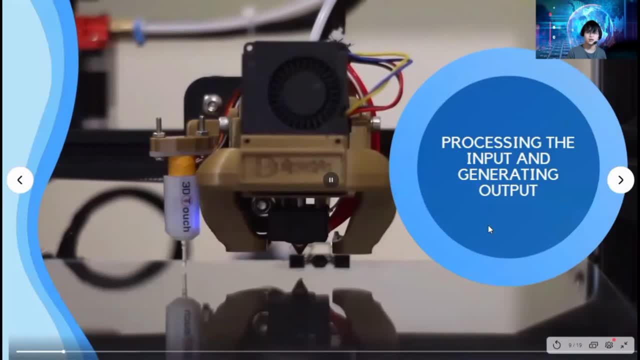 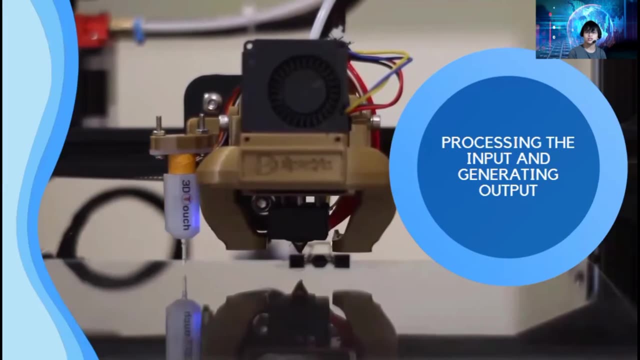 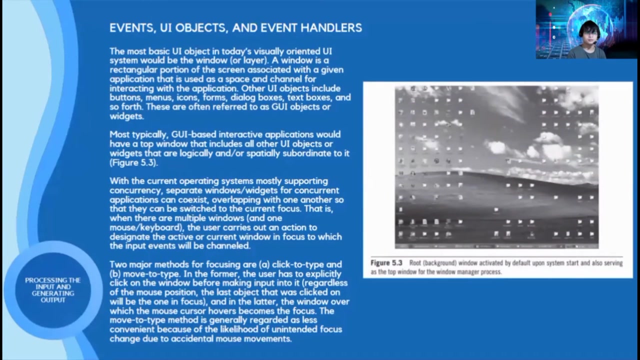 for efficient execution. ok, so that is the input and output at the low level. we hope that you get the concept on how computer works. now let's move forward on the processing and input: processing the input and generating the output. so how it happened, how it goes. okay, so first is we have the events, UI objects and event handlers. 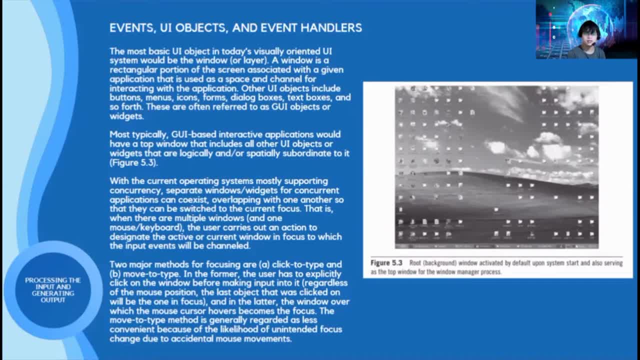 so how does it work? So the most basic UI object in today's visually-oriented UI system would be the window or layer. Sorry for my voice, guys. So a window is a rectangular portion of the screen associated with a given application that is used as space and channel for interacting with the applications. 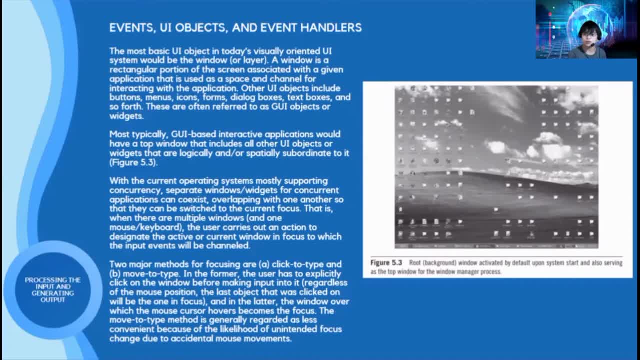 So other UI objects include- you know, you are familiar with the different buttons, menus, icons, forms, dialog boxes, text boxes and so forth, So these are often referred to as GUI objects or widgets. Okay, so it's very, you know, self-explanatory and you can comprehend it easily. 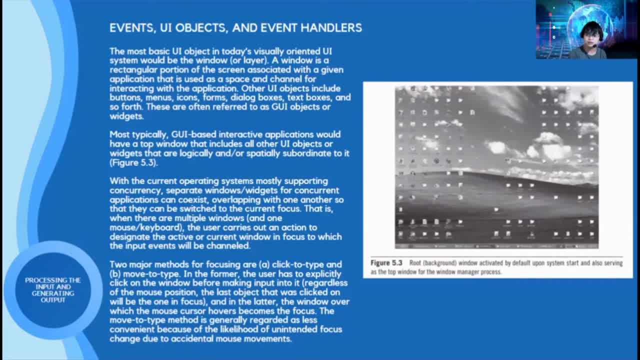 Most typically GUI-based interactive applications would have a top window that includes all other UI objects. So, as you can see in the figure 5.3, there are, you know, different widgets and UI objects. With the current operating systems, mostly supporting concurrency, separate window or widgets for concurrent applications can coexist. 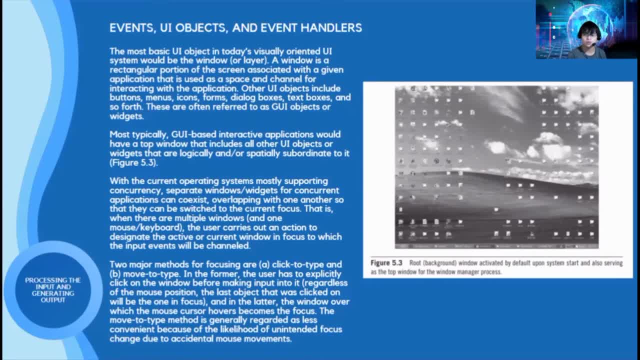 So overlapping with one another so that they can be switched to the current By another way of strumming this. for example, if you have multiple windows or other access tilts, you can check if some of the which are由 u tocar a auto or other album. use Auntie Pottery interpreter to locate an active or current window in focus in the upper right window of the view in the video. incomplete row. 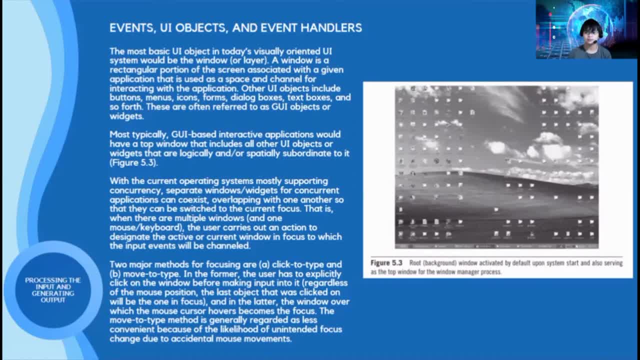 That is, when there are multiple windows and one mouse or keyboard. the user carries out an action to designate the active or current window in focus. the word menu of the display window is selected at a time or time where the input events are channeled by little checkboxes or key terus. 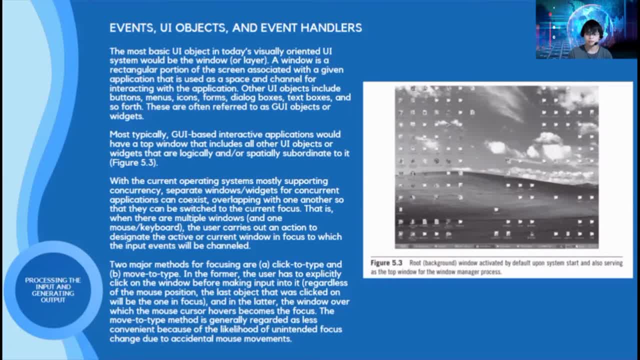 And we have this: two major events for focusing. First is the Click to type and then Move to Type: click on the window before making input into it. okay, regardless of the mouse position. so the last object that was clicked on on will be the one in focus and in the latter, the window over which the 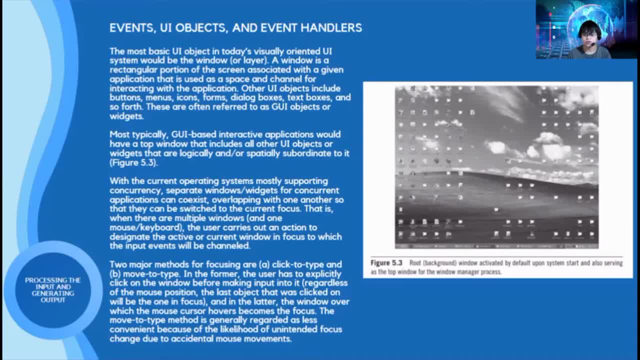 mouse cursor hovers becomes a focus. so the move to type method is generally regarded as less convenient because of likelihood of unintended focus change due to accidental mouse movements. okay, so again this figure. we have the root or the background window activated by default upon system start and also serving as the top window for the window manager process. so there are. 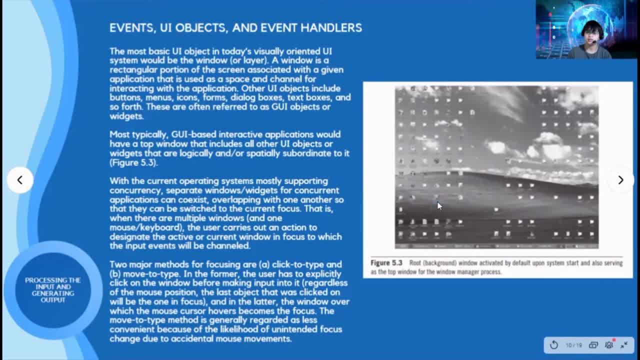 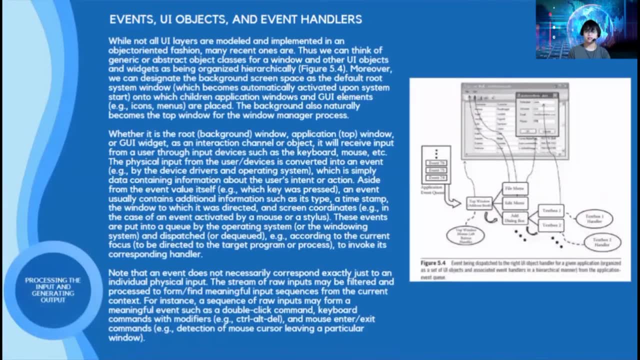 different. you know, you a object and different widgets. okay, so that is how it goes. okay, so for continuation, while not all you a layers are modeled and implemented in an object oriented fashion, many recent ones are. okay. this we can think of a generic or abstract object, classes for a window and other UI objects, and 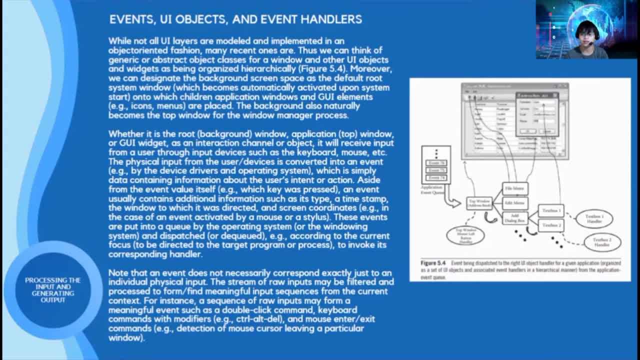 we as being organized errorically. so this one sample. moreover, we can designate the background screen space as the default root system window, which becomes automatically activated upon system start okay and to which children, application windows and go away elements icons been used are placed. so the background are also naturally becomes the top window for the window manager. 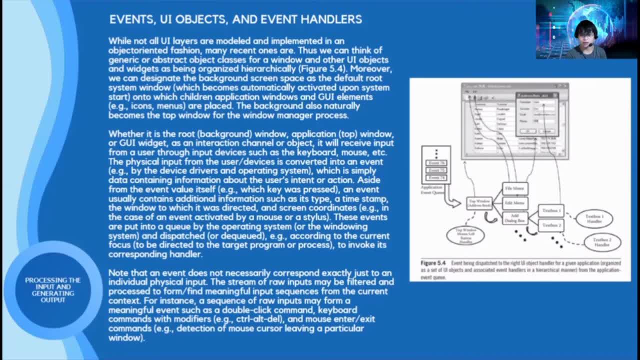 process okay. next, whether it is the root or background window, application or top window or go a widget as an interaction channel or object, it will receive input from a user through input devices such as keyboard, mouse etc. so the physical input from the user or devices is converted into an event. okay. 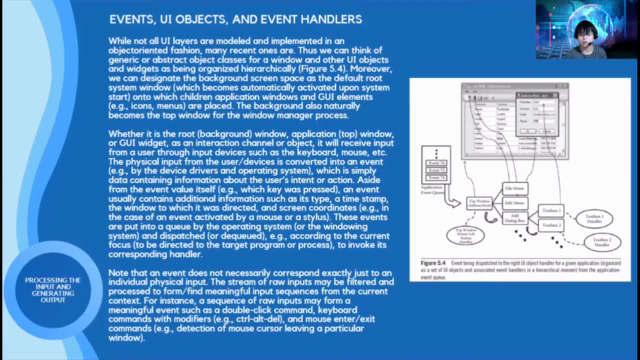 by the device, drivers and operating system, which is simply data containing information about the user's intent or action. so, aside from the event value itself, which you know- K was pressed or etc. an event usually contains additional information such as the type, you know, a timestamp and the window to which it was directed. 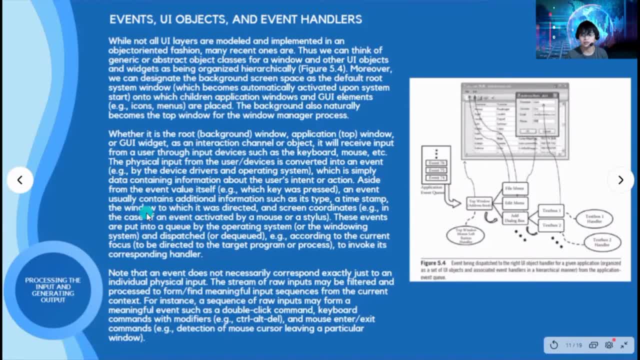 and screen coordinates sample in the case of an event activated by a mouse or stylus. so these events are put into queue where the operating system or the windowing system and dispatched, or the queue now according to the current focus, so to be directed to the target program or process to involve its corresponding 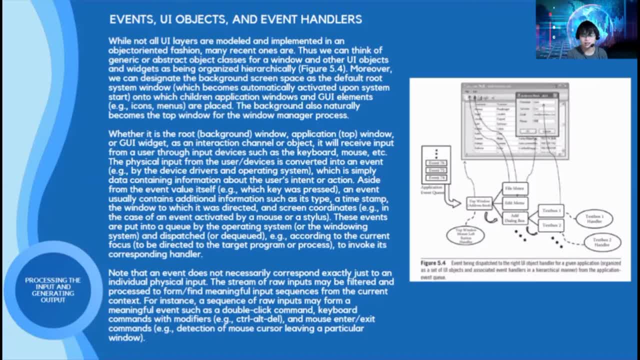 handler. okay, so note that an event does not necessarily correspond exactly just one individual physical input. so the stream of row inputs may be filtered and process to form find meaningful input sequences from the current context. okay, so for instance, a sequence of you know row inputs may form meaningful events. 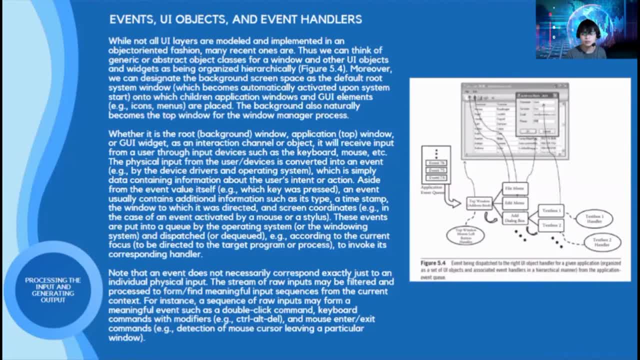 such as a double key command, keyboard commands with modifiers and a mouse enter or exit command, so the detection of mask cursor, leaving a particular window. so okay, so to simply summarize it, guys, you know, when you give instructions to computer, it will generate a signal, no, an interrupt signal. 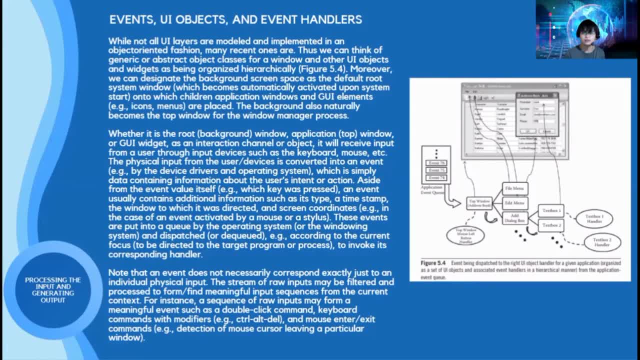 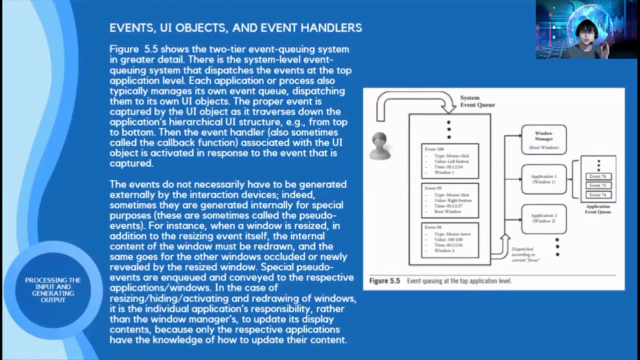 it will gonna say to the CPU that there's process, now there's an instruction given by a user and then, yeah, it will be processed. okay, next we have: okay, let's continue with this diagram. okay, let's continue with this diagram. okay, let's continue with this diagram. so the this figure shows that the 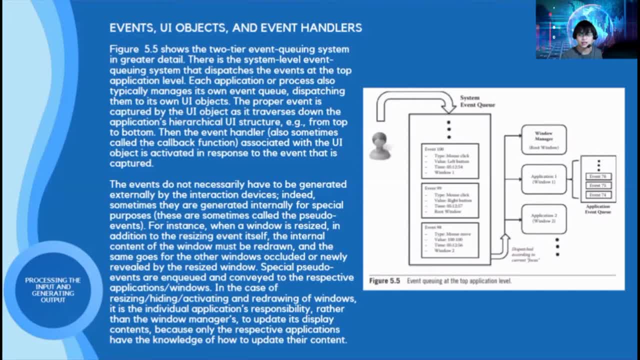 so the this figure shows that the. so the this figure shows that the two-tier event queuing system is created. two-tier event queuing system is created. two-tier event queuing system is created in greater detail. okay, so there is the. in greater detail. okay, so there is the. 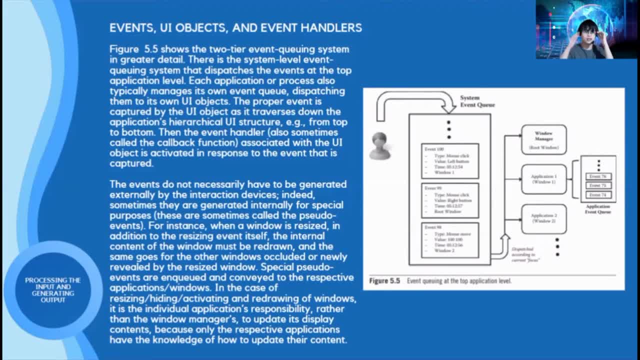 in greater detail. okay, so there is the system level event queuing system, that system level event queuing system, that system level event queuing system that dispatch the events at the top of the dispatch, the events at the top of the dispatch, the events at the top of the application level, and each application or 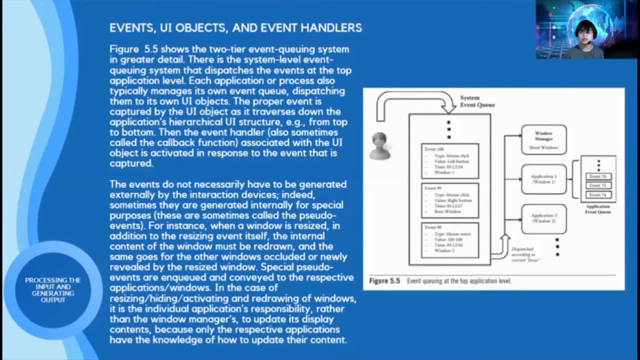 application level and each application or application level and each application or process also. typically you know manage process also. typically you know manage process also. typically you know manage its own event queue, dispatching them to its own event queue, dispatching them to its own event queue, dispatching them to its own UI objects- okay, so I hope that. 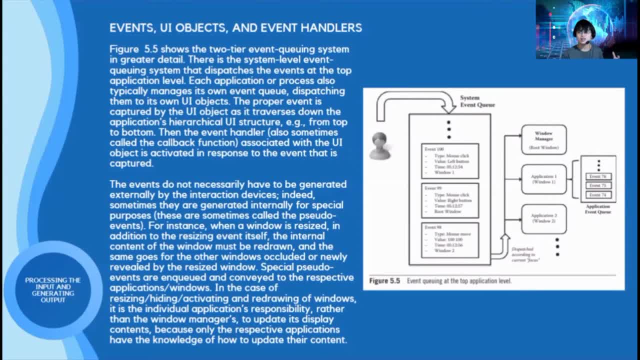 its own UI objects okay, so I hope that its own UI objects okay. so I hope that you are, you know, currently gonna, you are, you know, currently gonna. you are, you know, currently gonna imagine in your own cigar heatable. so, imagine in your own cigar heatable. so 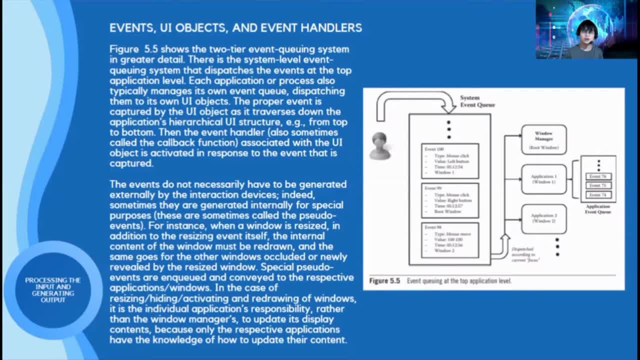 imagine in your own cigar heatable. so yeah, so the proper event is captured by. yeah, so the proper event is captured by. yeah, so the proper event is captured by the UI object as it traverses down the. the UI object as it traverses down the, the UI object as it traverses down the application's hierarchical UI structure. 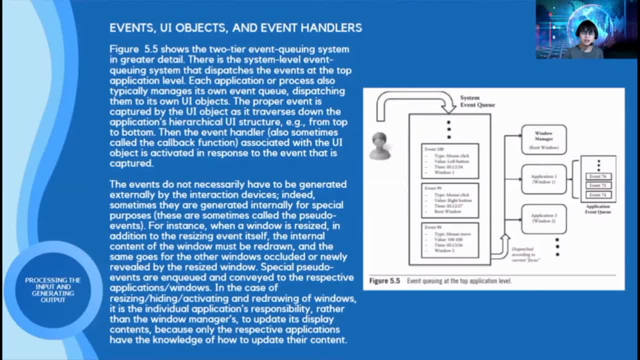 application's hierarchical UI structure. application's hierarchical UI structure: okay, from the top to bottom. then the okay from the top to bottom. then the okay from the top to bottom. then the event handler, also sometimes called the event handler, also sometimes called the event handler, also sometimes called the callback function. functions associated: 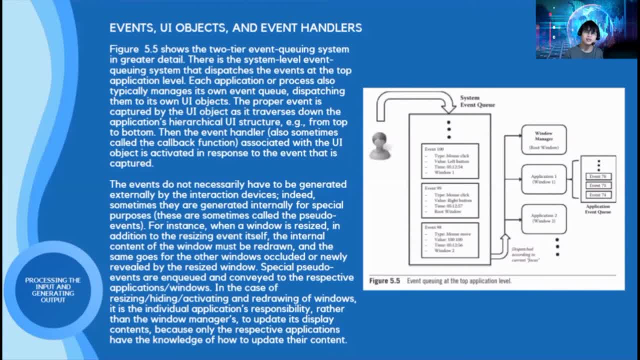 callback function functions- associated callback function functions associated with the UI object is activated in with the UI object is activated in with the UI object is activated in response to the event that is capturing. response to the event that is capturing. response to the event that is capturing. okay, so the events do not necessarily 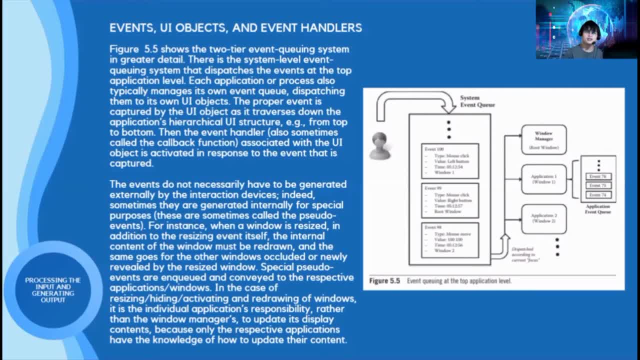 okay. so the events do not necessarily okay. so the events do not necessarily have to be generated externally by the have to be generated externally by the have to be generated externally by the interaction devices. indeed, sometimes interaction devices, indeed, sometimes interaction devices, indeed, sometimes they are generated internally, for 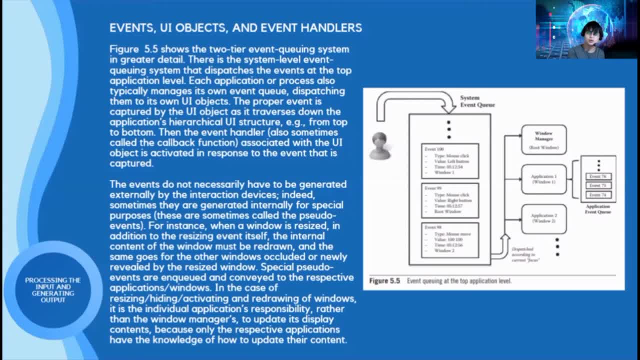 they are generated internally, for they are generated internally for special purposes, so these are sometimes special purposes, so these are sometimes special purposes, so these are sometimes called the pseudo events. so for instance called the pseudo events. so for instance called the pseudo events. so for instance, when a window is resized in addition, 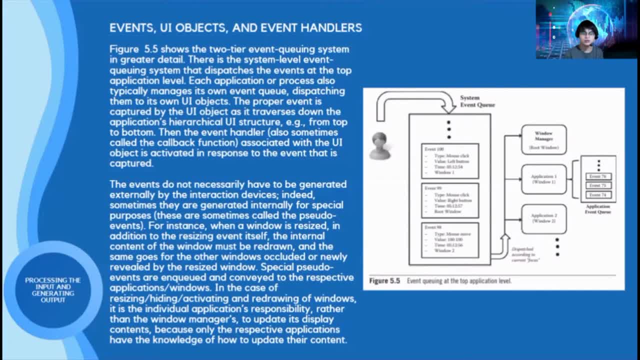 when a window is resized. in addition, when a window is resized, in addition to the resizing event itself, the internal to the resizing event itself, the internal to the resizing event itself, the internal content of the window must be redrawn. content of the window must be redrawn. 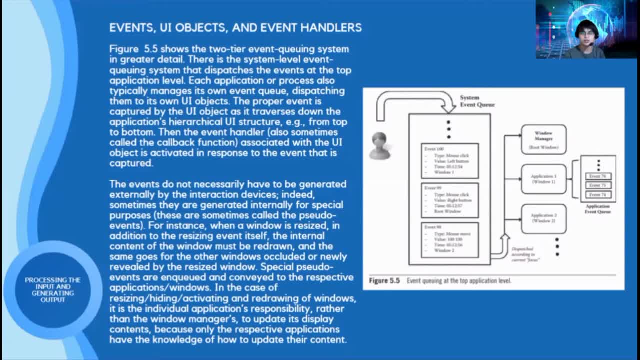 content of the window must be redrawn in the same goals for the other windows, in the same goals for the other windows, in the same goals for the other windows, occluded or newly revealed by the occluded or newly revealed by the occluded or newly revealed by the resized window. okay, so special sort of 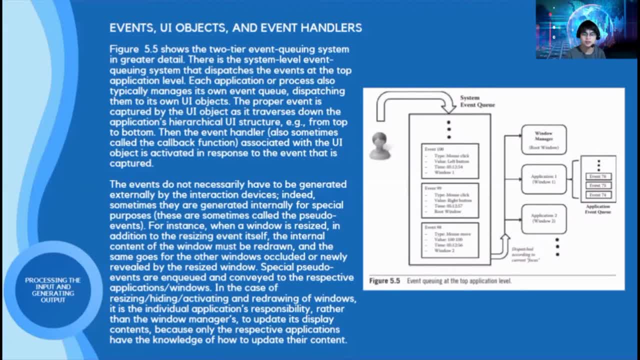 resized window. okay, so special sort of resized window. okay, so special sort of code. so the events are in cute and code. so the events are in cute and code. so the events are in cute and conveyed to the respective applications, or conveyed to the respective applications. or conveyed to the respective applications or windows in the case of resizing. or. 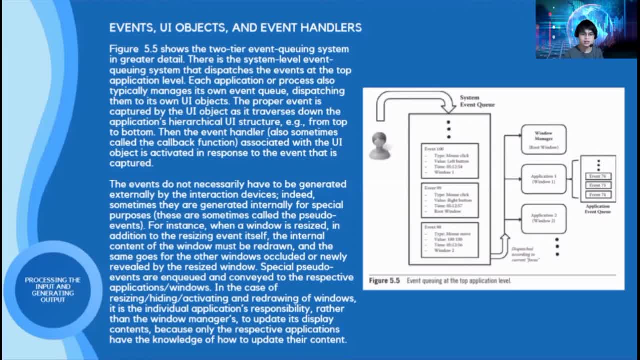 windows in the case of resizing, or windows in the case of resizing or hiding or activating and redrawing of hiding or activating and redrawing of hiding or activating and redrawing of windows. it is in the. it is the individual windows. it is in the. it is the individual. 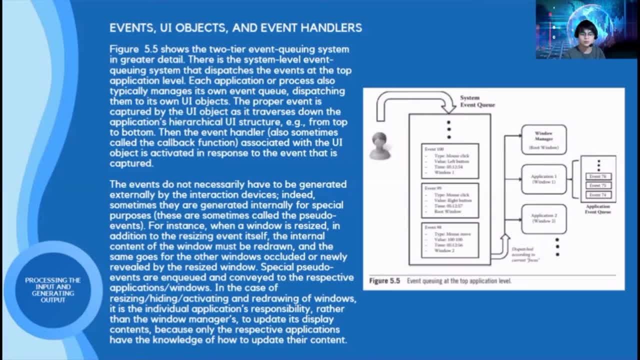 windows, it is in the, it is the individual applications responsibility, rather than applications responsibility, rather than applications responsibility, rather than the windows managers to update its, the windows managers to update its, the windows managers to update its display contents, because the respective display contents, because the respective display contents, because the respective applications have the knowledge on how. 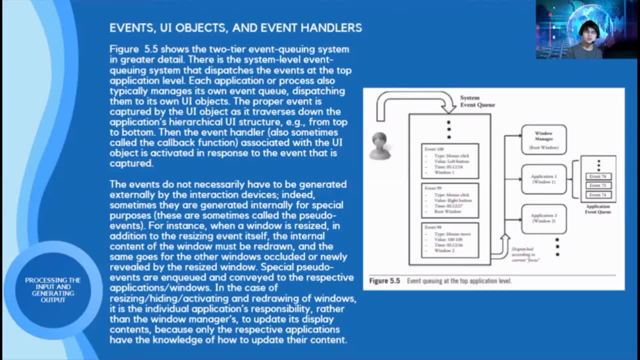 applications have the knowledge on how. applications have the knowledge on how, of how to update their content. okay, so I, of how to update their content. okay, so I, of how to update their content. okay, so I think if you actually read it again, it's think if you actually read it again, it's. 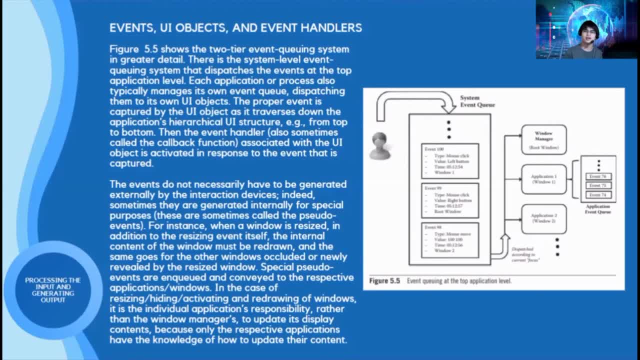 think if you actually read it again, it's very you know self-explanatory and you very you know self-explanatory and you very you know self-explanatory and you can grasp the idea and what is happening, can grasp the idea and what is happening. 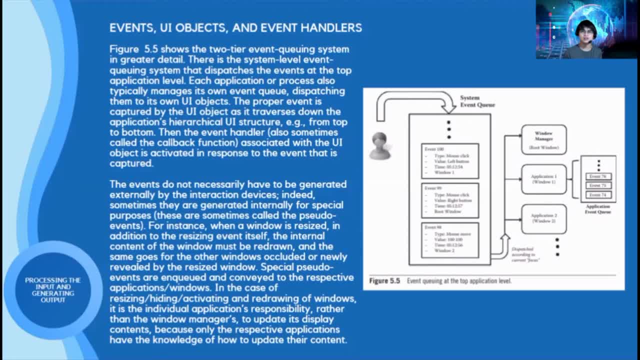 can grasp the idea and what is happening. know what is happening with the different. know what is happening with the different. know what is happening with the different events how it was created. you know the events how it was created. you know the events how it was created. you know the different UI objects and what are the. 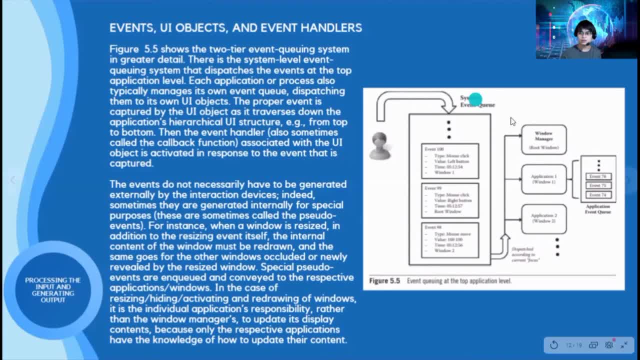 different UI objects and what are the different UI objects and what are the different event handlers. okay, so this is different event handlers. okay, so, this is different event handlers. okay, so this is what the diagram is. you know telling you what the diagram is. you know, telling you. 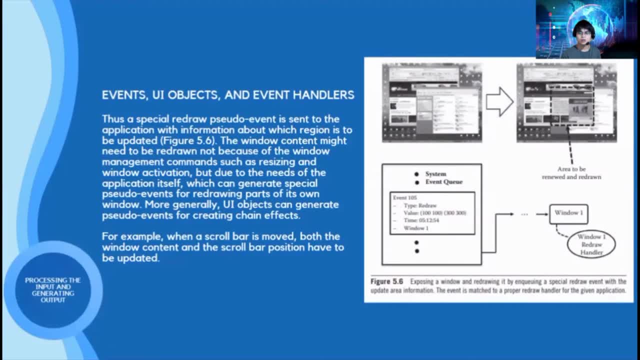 what the diagram is. you know telling you, and yeah, so this figure, okay, this is. and yeah, so this figure, okay, this is. and yeah, so this figure, okay, this is another. you know sample, so there's a another. you know sample, so there's a another. you know sample, so there's a special. we draw so the code. pseudo event. 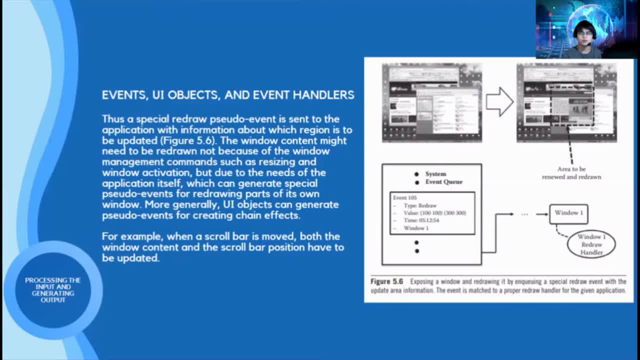 special we draw. so the code pseudo event: special we draw. so the code pseudo event is sent to the application with the is sent to the application with the is sent to the application with the information about which region is to be. information about which region is to be. 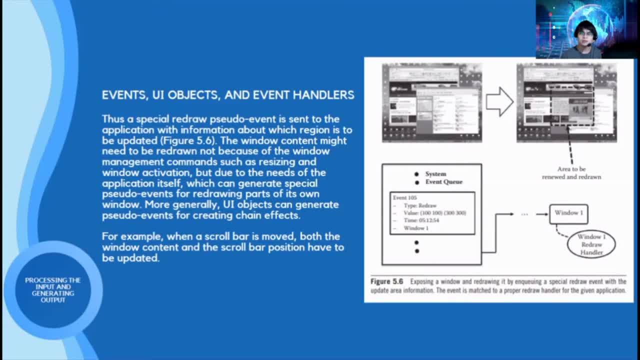 information about which region is to be updated. okay, so the window content might updated. okay, so the window content might updated. okay, so the window content might be need to be redrawn. not because of the be need to be redrawn, not because of the be need to be redrawn, not because of the window management commands, such as: 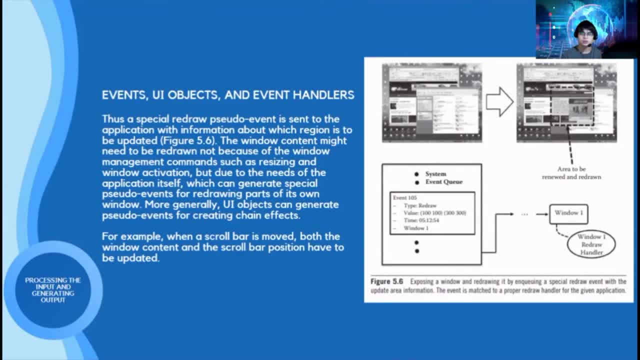 window management commands, such as window management commands, such as resizing, and you know window activation, resizing and you know window activation, resizing and you know window activation, but due to the needs of the application, but due to the needs of the application, but due to the needs of the application itself. 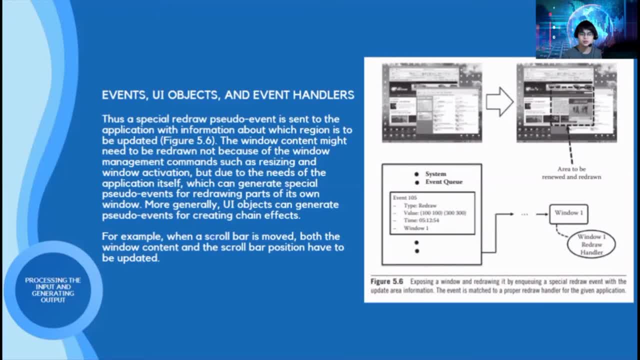 itself itself, which can be generate, which can generate, which can be generate, which can generate, which can be generate, which can generate. special pseudo events for redrawing, special pseudo events for redrawing, special pseudo events for redrawing parts of its own window more generally, parts of its own window more generally. 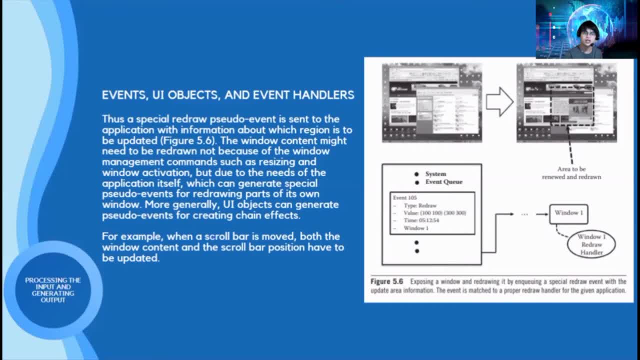 parts of its own window. more generally, ui objects can generate soda events of ui objects can generate soda events of ui objects can generate soda events of creating, creating, creating chain effects. so, for example, when a chain effects. so, for example, when a chain effects. so, for example, when a scroll bar is moved, both the window. 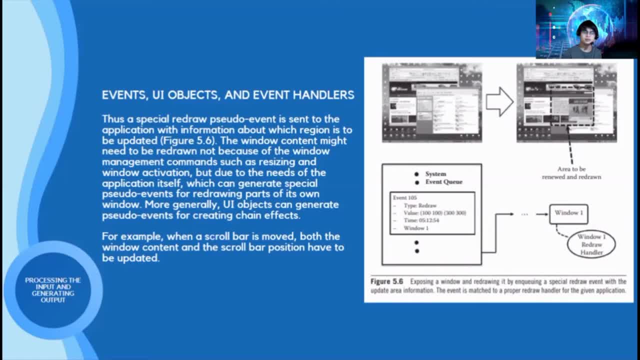 scroll bar is moved. both the window scroll bar is moved. both the window content and the scroll bar position have content and the scroll bar position have content and the scroll bar position have to be updated. so um will not you know to be updated. so um will not you know. 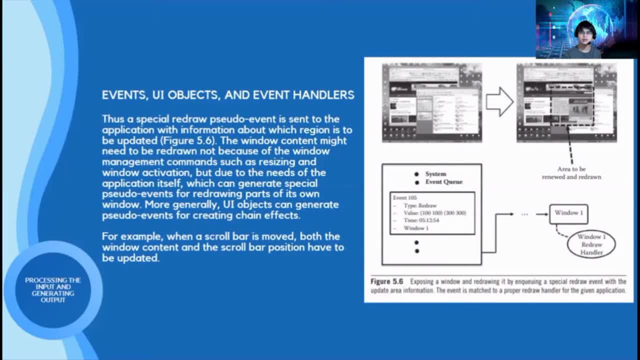 to be updated. so um will not, you know, go through everything about programming. go through everything about programming. go through everything about programming, how it is being programmed, all you just how it is being programmed. all you just how it is being programmed. all you just do is to get the idea on. on the process. 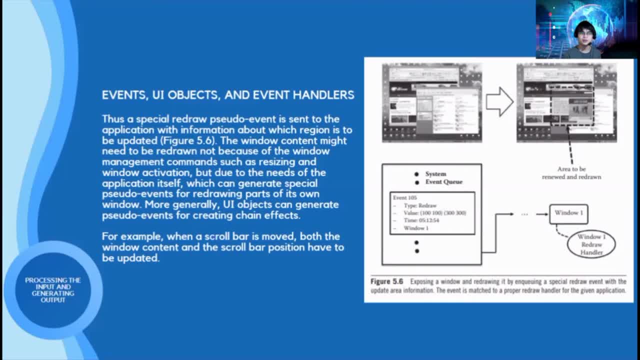 do is to get the idea on on the process. do is to get the idea on on the process, on how it happens. no, on how the input is on how it happens. no on how the input is on how it happens. no on how the input is being processed and how. 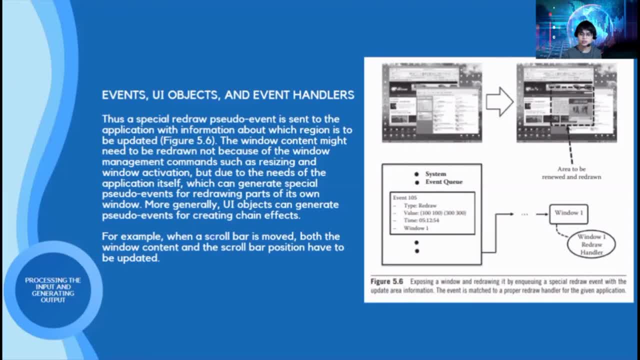 being processed and how being processed and how it is how the output is, how output is. it is how the output is how output is. it is how the output is, how output is being generated, being generated, being generated. okay, so when you give instructions to the, okay, so when you give instructions to the 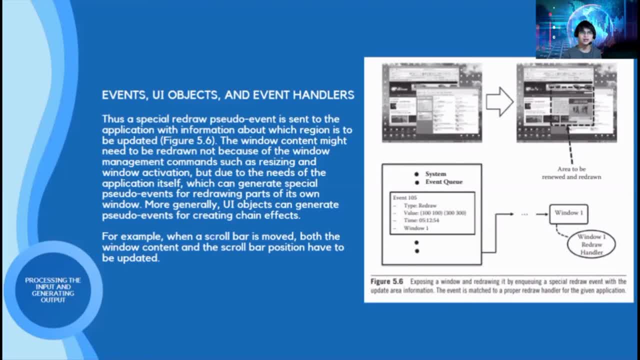 okay. so when you give instructions to the user, user, user- then there it sends, then there it sends, then there it sends, you know. signal to the cpu, the cpu will you know. signal to the cpu. the cpu will you know. signal to the cpu. the cpu will win the process. 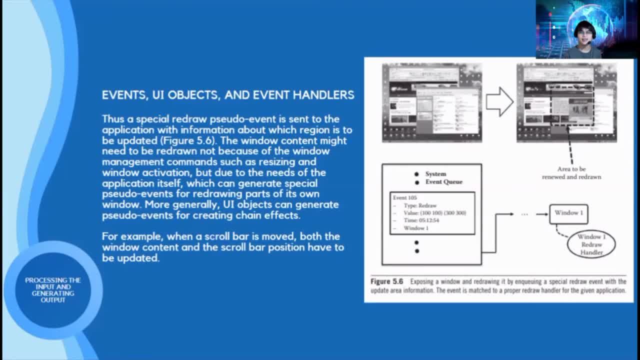 win the process. win the process. there is queuing, you know there is queuing, you know there is queuing, you know, and then you know it will then generate, and then you know it will then generate, and then you know it will then generate the output. so i hope. 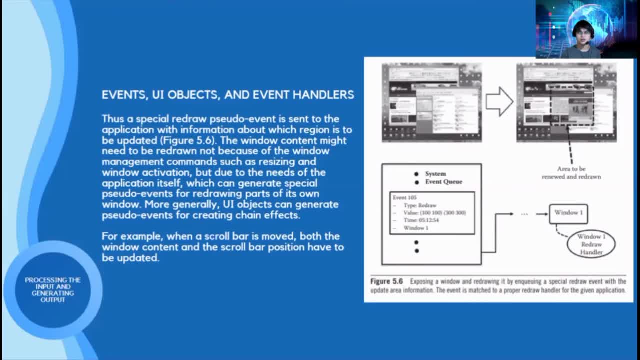 the output. so i hope the output. so i hope you guys get the idea on how it is being. you guys get the idea on how it is being, you guys get the idea on how it is being processed, processed, processed, um in your gonna imagine, um in your gonna imagine. 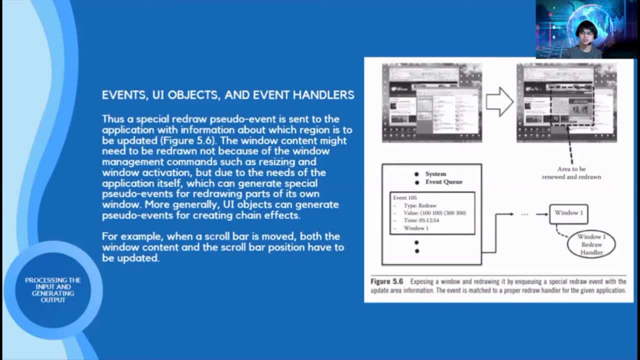 um, in, your gonna imagine you're going to see it on the computer. you're going to see it on the computer. you're going to see it on the computer now when you give instructions to it, now, when you give instructions to it, now when you give instructions to it. okay, 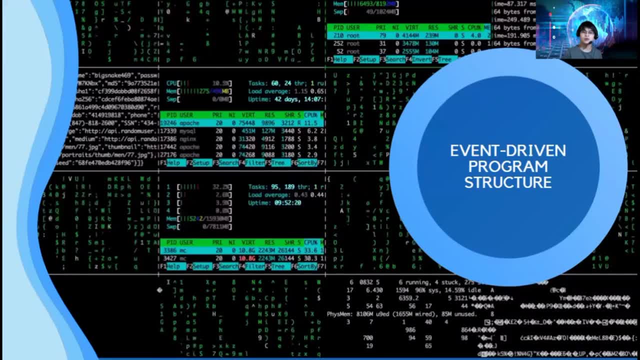 okay, okay, okay, so we'll move forward with the event. okay, so we'll move forward with the event. okay, so we'll move forward with the event driven program structure driven program structure. driven program structure. okay, what is this structure? don't worry. okay, what is this structure? don't worry. 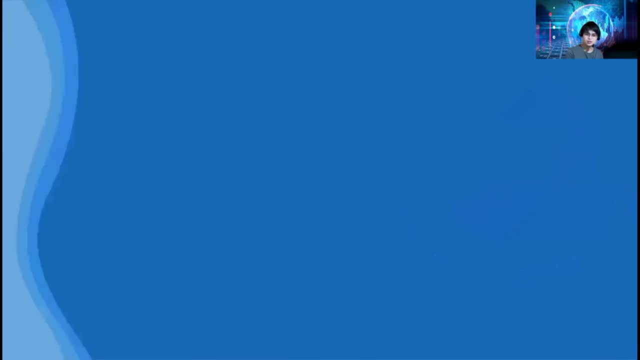 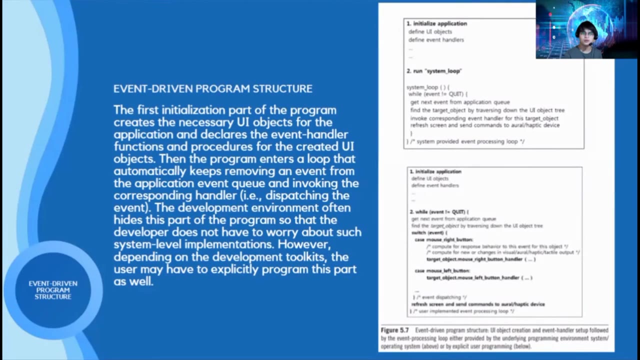 okay, what is this structure? don't worry, okay, um, okay, um, okay, um okay, so the event driven program. okay, so the event driven program. okay, so the event driven program structure. structure. structure: the first initialization part of the. the first initialization part of the. the first initialization part of the program creates the necessary ui objects. 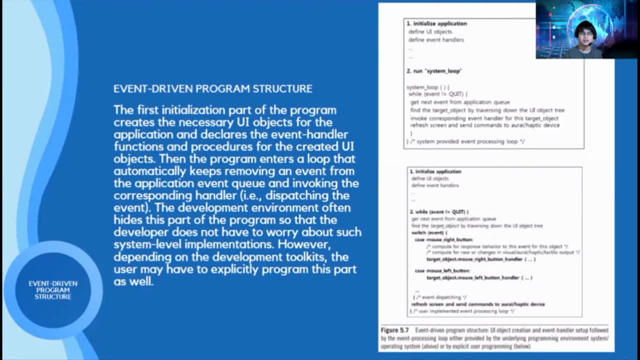 program creates the necessary ui objects. program creates the necessary ui objects and declares the event handler. and declares the event handler and declares the event handler. functions and procedures. functions and procedures. functions and procedures for the created ui objects. okay, so then, for the created ui objects. okay, so then. 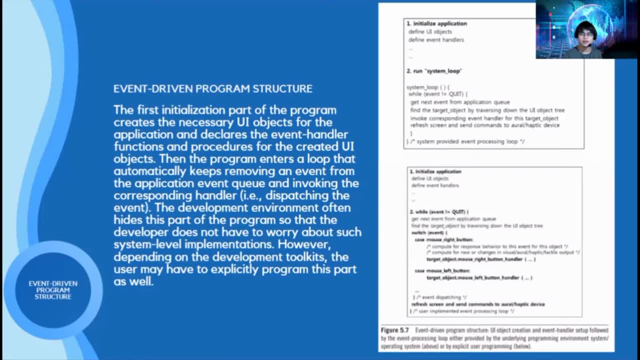 for the created ui objects. okay, so then the program enters a loop, that the program enters a loop, that the program enters a loop that automatically keeps removing an event, automatically keeps removing an event, automatically keeps removing an event from the application event queue and from the application event queue, and 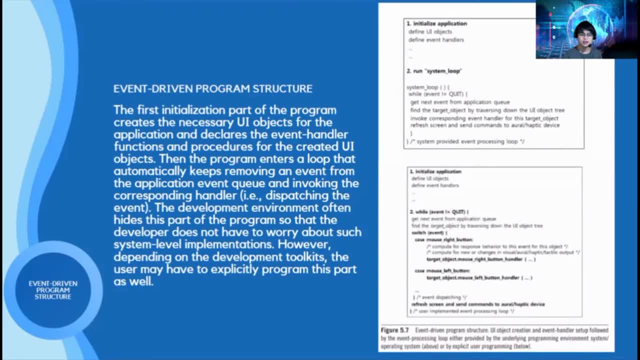 from the application event queue and invoking the corresponding handler. invoking the corresponding handler. invoking the corresponding handler, dispatching- the you know dispatching the dispatching, the you know dispatching the dispatching, the you know dispatching the event, event, event. so the development environment often. so, the development environment often. 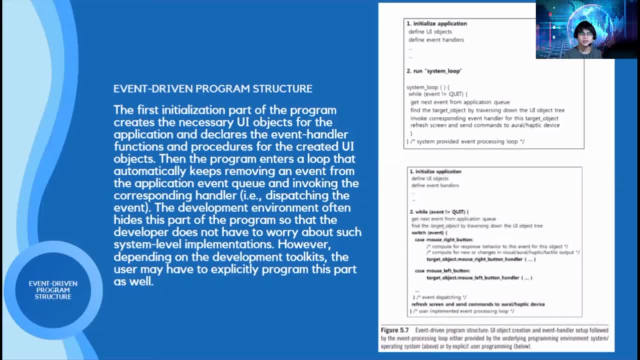 so the development environment often hides this part of the program. so the development environment often hides this part of the program so that the developer does not have to, so that the developer does not have to, so that the developer does not have to worry about worry about worry about such system level implementations. 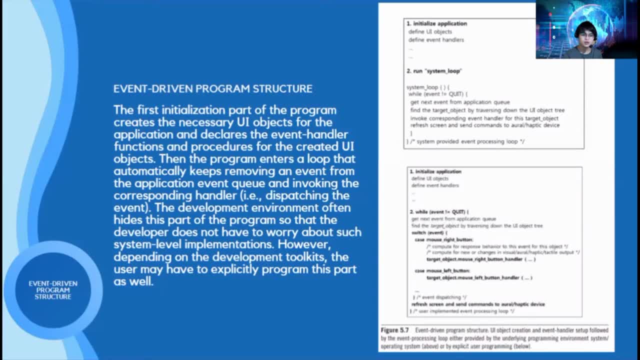 such system level implementations, such system level implementations, however, depending on the development. however, depending on the development, however, depending on the development toolkit, toolkit, toolkit. the user may have to explicitly program. the user may have to explicitly program. the user may have to explicitly program this part as well. 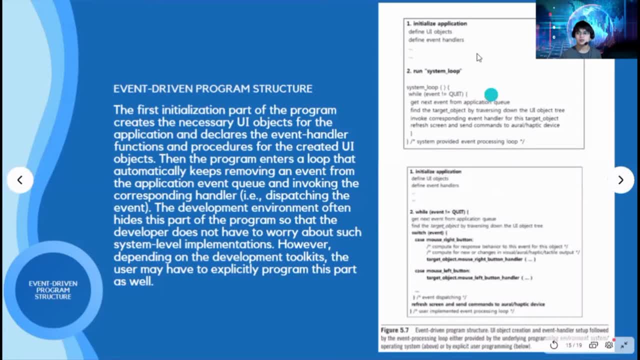 this part as well, this part as well. so, um, this, this one is the sample part. so, um, this, this one is the sample part. so, um, this, this one is the sample part. this is actually a job of a developer. this is actually a job of a developer. 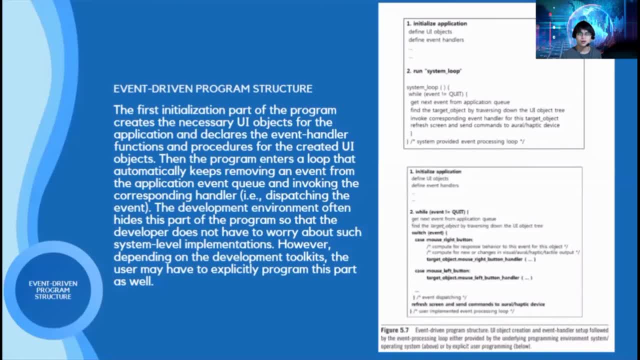 this is actually a job of a developer, but i just like you to you know, see, but i just like you to you know, see, but i just like you to you know see what, how? no, you know what, how no, you know what, how no, you know. okay, actually, um, what happens is 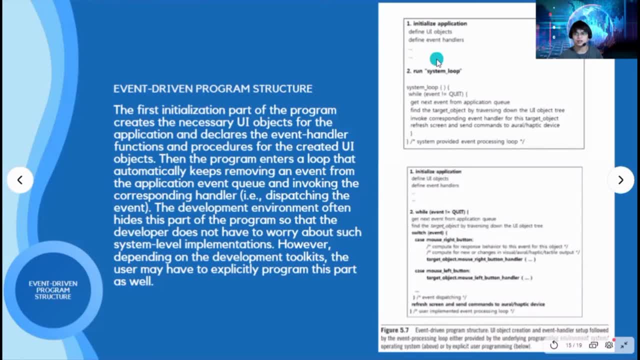 okay, actually, um, what happens is okay, actually, um, what happens is: you know we. you initialize the application. you know we. you initialize the application. you know we. you initialize the application, you define the different ui objects, you define the different ui objects, you define the different ui objects, you define the event huddlers and then 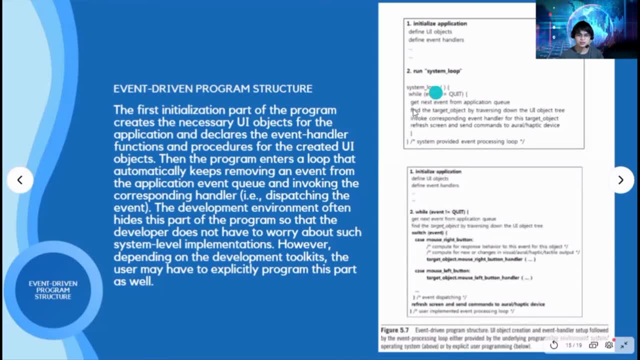 you define the event huddlers and then you define the event huddlers and then you run the system loop. so there are, you run the system loop. so there are, you run the system loop. so there are different, different, different, you know functions, and then, yeah, 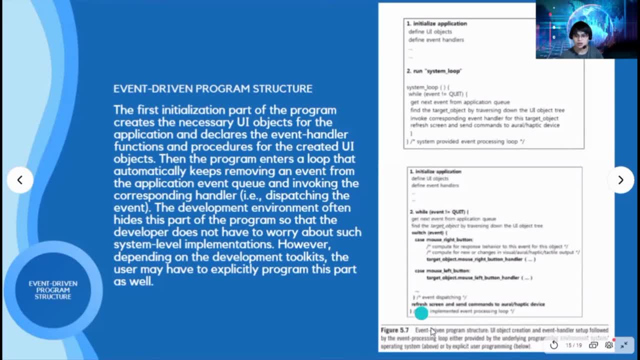 you know functions and then, yeah, you know functions, and then, yeah, you sloop. and then the last one is you sloop, and then the last one is: you know, you refresh the screen and send you know you refresh the screen and send you know you refresh the screen and send commands to oral or haptic device. 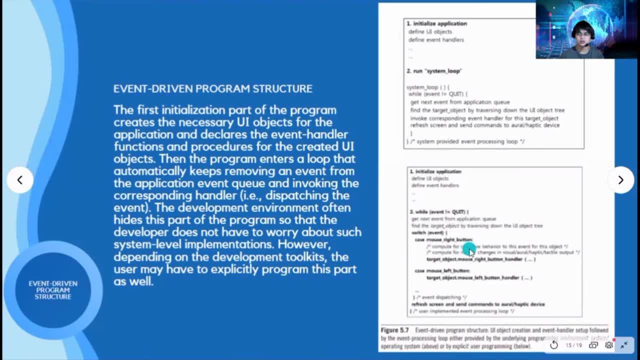 commands to oral or haptic device. commands to oral or haptic device. so this one is the the structure, so this one is the the structure, so this one is the the structure. okay, so again on, so you write a book you. okay, so again on, so you write a book you. 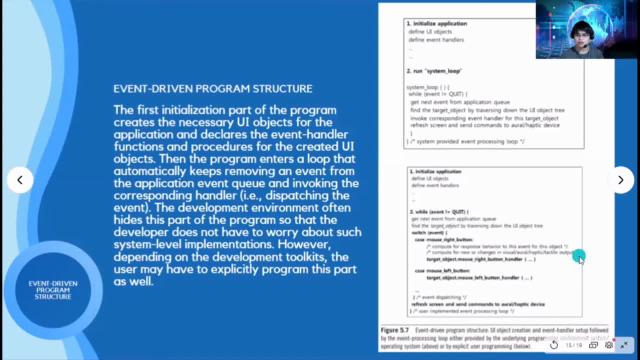 okay, so again on. so you write a book. you, in a light, initialize the application. in a light, initialize the application in a light, initialize the application. you run the system loop. okay, you run the system loop. okay, you run the system loop. okay, so don't worry. okay, dealing with the. 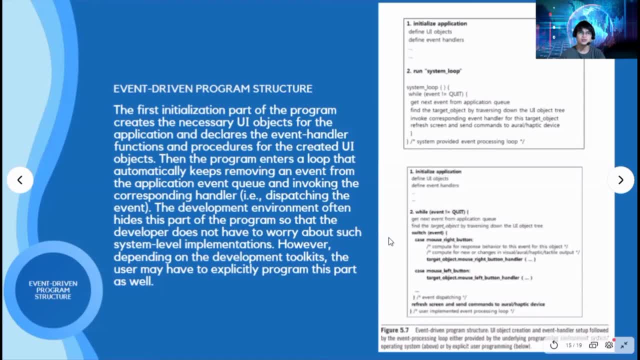 so don't worry, okay, dealing with the. so don't worry, okay, dealing with the program now. program now. program. now we're not going to, you know um, we're not going to, you know um, It has a lot of topics, okay, Just get the structure of the program, okay. 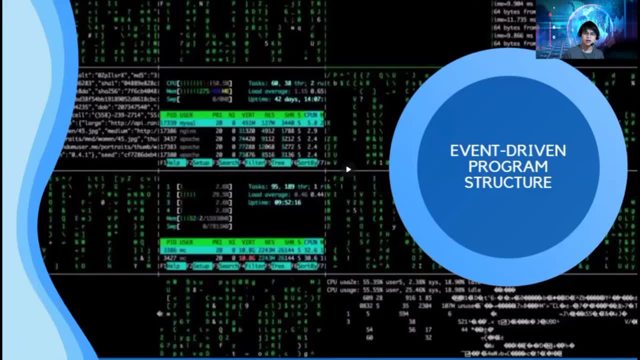 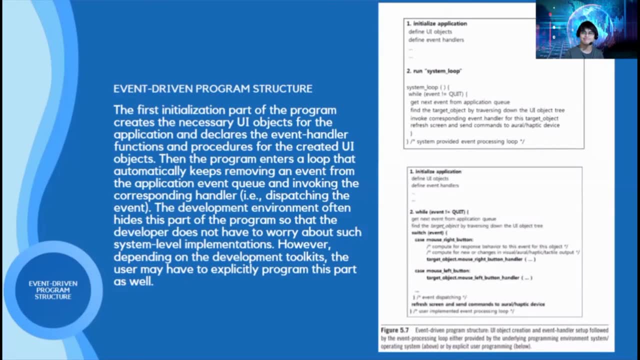 I hope that you are learning so far. So that's it. That is how the event-driven program. that is just the structure, no Of the event-driven program. okay, So it depends on which programming language you are going to use. 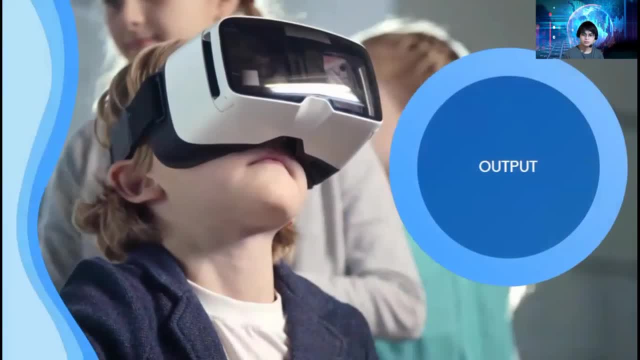 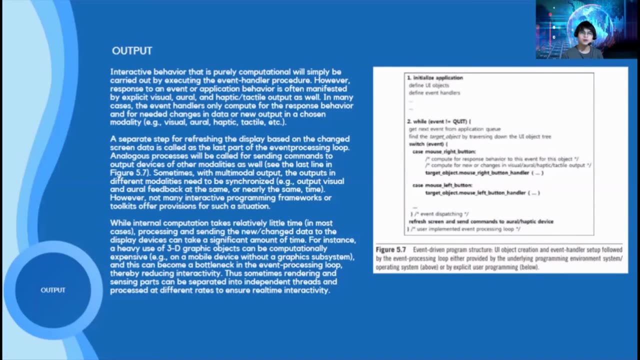 Okay, next is the output. So we'll discuss the output. So the output- of course, interactive behavior that is purely computational, will simply be carried out by executing the event handler procedure. However, response to an event or application behavior is often manifested by explicit, visual, oral and haptic tactile output as well. 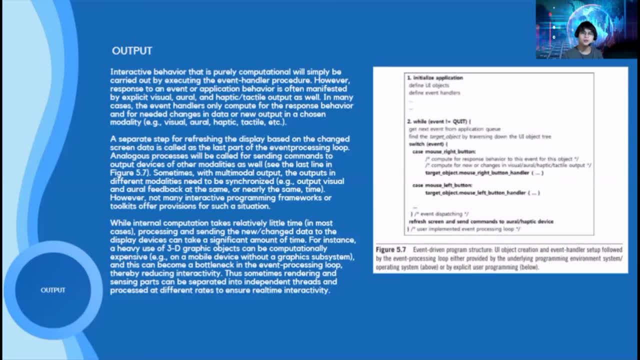 So in many cases the event handlers only compute for the response behavior and for needed changes in data or new output in a chosen modality: visual, oral, haptic, tactile, etc. I know that you have an idea about, you know visual, oral, haptic and tactile from the previous chapter. 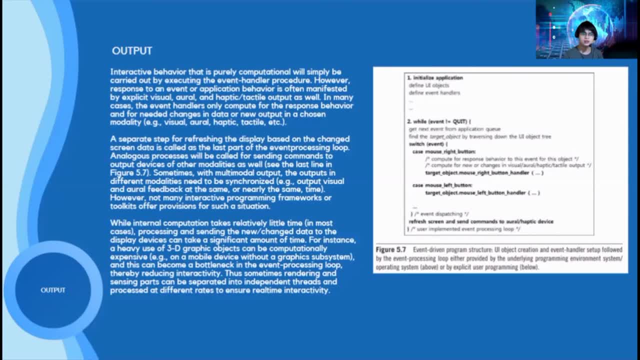 So a separate step for refreshing the display based on the change screen. data is called. data is called as the last part of a second part of the event processing loop, So analogous processes will be called for, sending commands to the output devices of the other modalities as well. 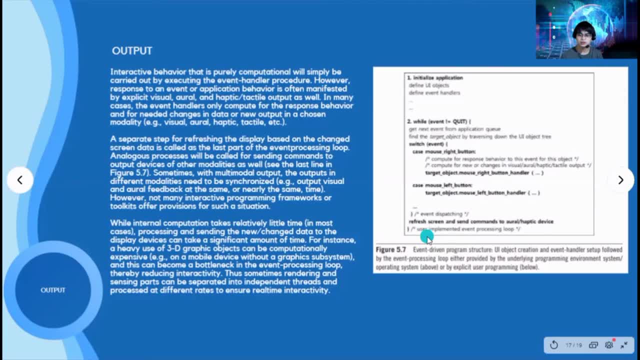 So this one is the sample. no, It refreshes screen and send commands to oral or haptic device. So sometimes with multi-modal output, the output is in different modalities need to be synchronized. Okay, output visual and oral feedback at the same time. 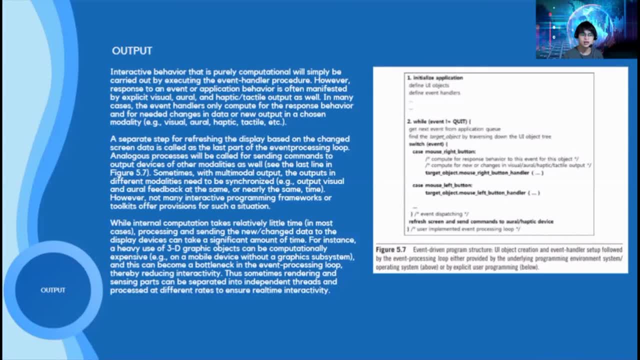 you know at the same time, the same or nearly the same time. So, however, not many interactive programming frameworks or toolkits offer provisions for such a situation. So, while internal computation takes relatively little time in most cases, processing and sending the new, changed data. 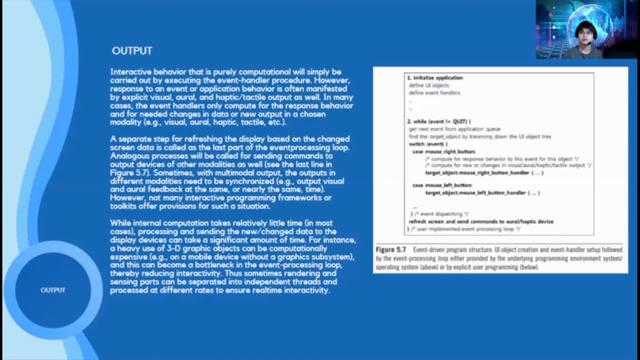 to the display devices can take a significant amount of time. So, for instance, a heavy use of 3D graphic objects can be computationally expensive. So on, mobile device without graphic subsystem, and this can become a bottleneck in the event processing loop. 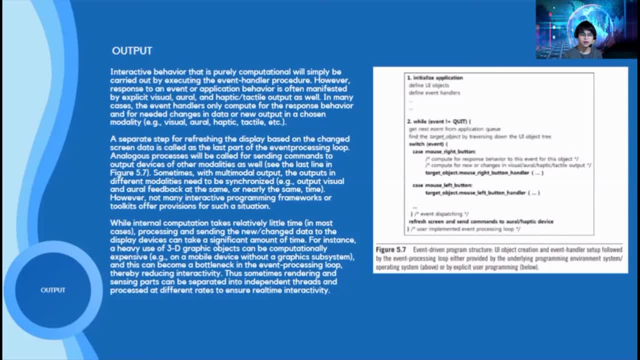 thereby reducing interactively The sometimes rendering and sensing parts can be separated into independent threads and process at different rates to ensure real time interactively. So that is how the output is being generated. OK, So again, if listed cases have done, just re-read again. 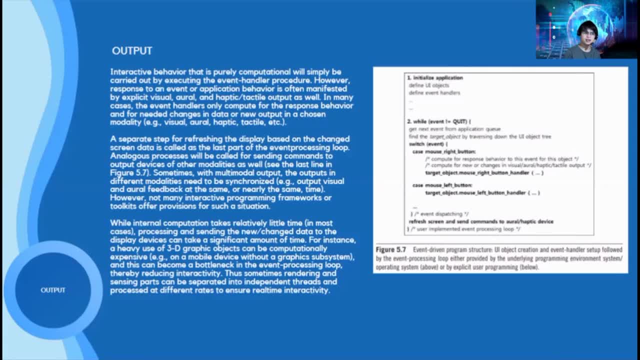 And you can see what the process looks like. Now, output. right, It is the one which is, you know, you are viewing in your screen. When you give instructions to the users, when you give the inputs, it's just going to give us output. 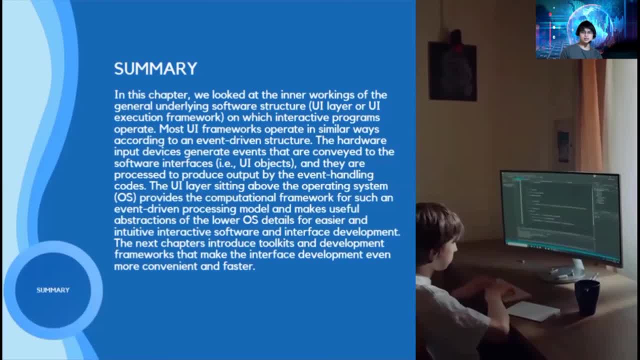 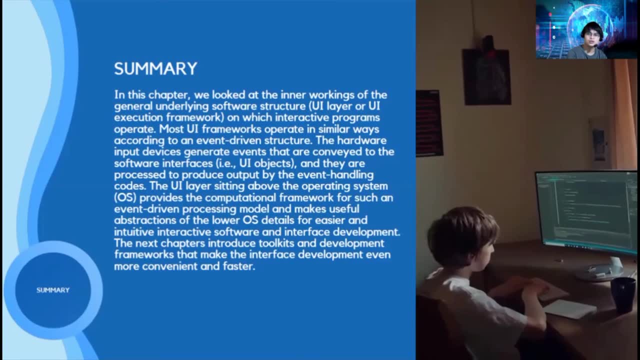 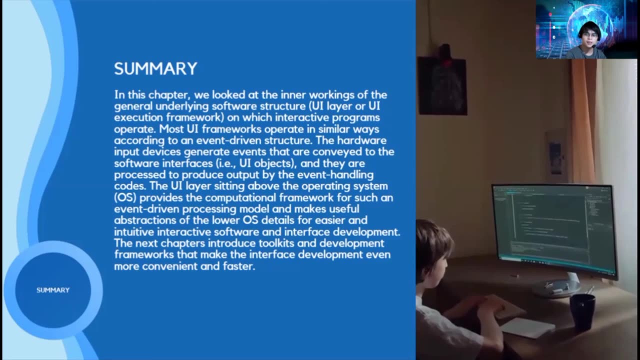 OK, Next. OK, So we are now in the summary. So in this chapter we looked at the inner workings of the general underlying software structure, UI layer or UI execution framework- on which interactive programs operate. So most UI frameworks operate in similar ways. 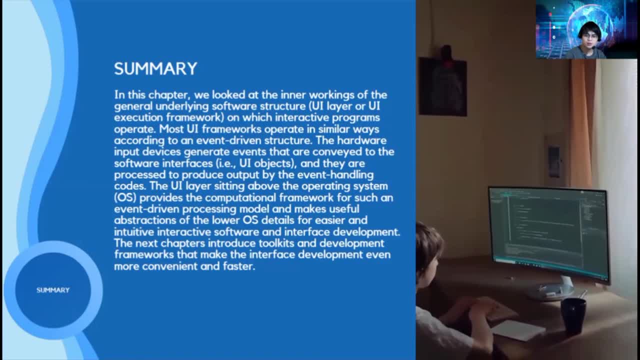 according to an event-driven structure. So the hardware input devices generate events that are conveyed to the software interfaces or UI objects, And they are generated, They are processed to produce output by the event-telling codes, Then the UI layer setting about the operating system or OS. 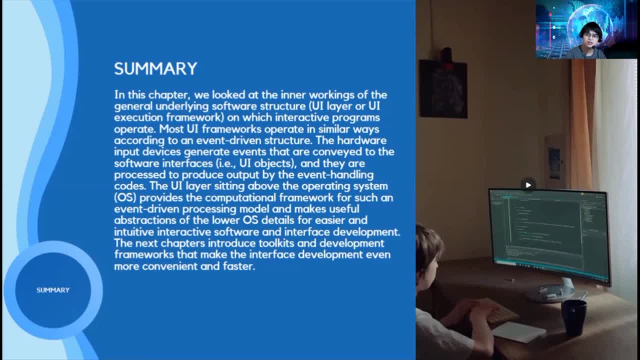 provides the computer's computational framework for such an event-driven processing model and makes useful abstractions of the lower OS details for easier and intuitive interactive software and interface development. And the next chapters introduce toolkits and development frameworks. These are the tools that make the interface development even.